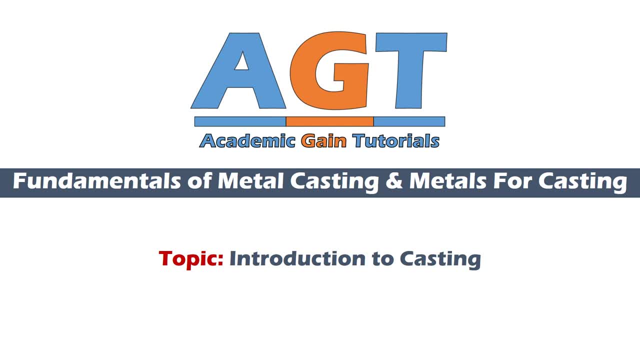 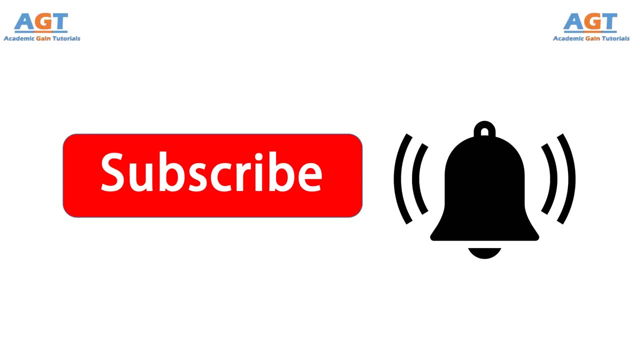 Welcome to Academic Game Tutorials. The topic of today's class is Introduction to Casting. We are studying Fundamentals of Metal Casting and Metals for Casting. We will cover all related topics one by one Before starting. if you haven't subscribed to this channel yet, just click on subscribe and press the bell icon. 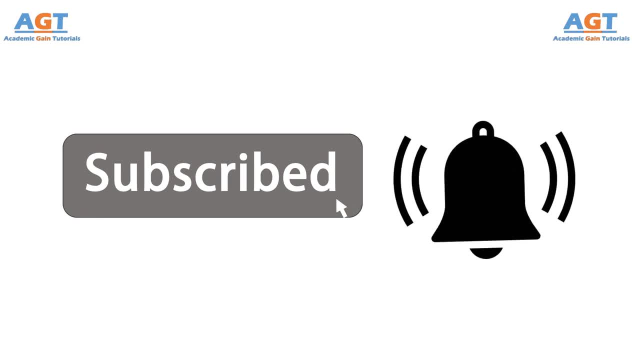 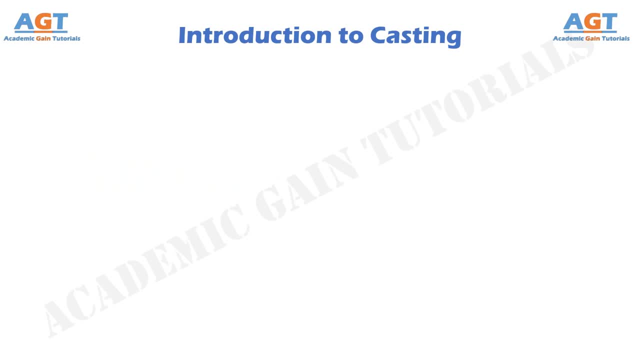 Here we come up with new videos on different subjects to make the academic studies easier for you. So into the topic. What is Casting? In casting, the starting work material is either a liquid or is in a highly plastic condition, and a part is created through solidification of the material. 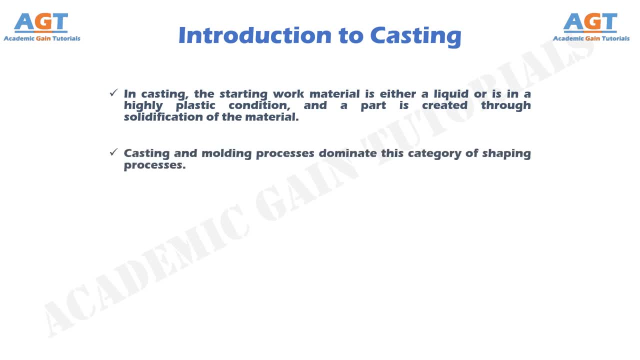 Casting and molding processes dominate this category of shaping processes. The solidification processes can be classified according to engineering material being processed, That is, solidification of metals, Solidification of ceramics, Specifically glasses, And the solidification of polymers and polymer matrix composites, or in short, PMCs. 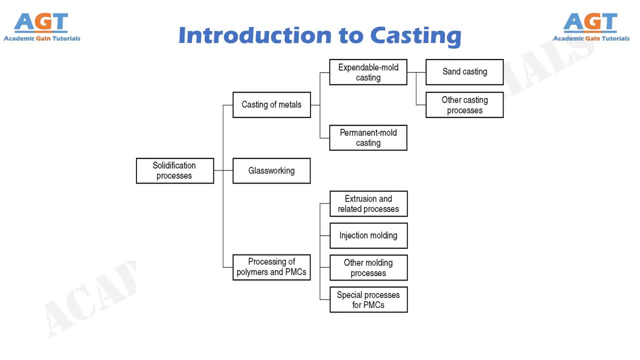 So during casting, the solidification processes can be classified into three types, depending on which type of material is being processed, That is, casting of metals, glassworking and processing of polymers and PMCs, or the polymer matrix composites. The casting of metals can be further classified. 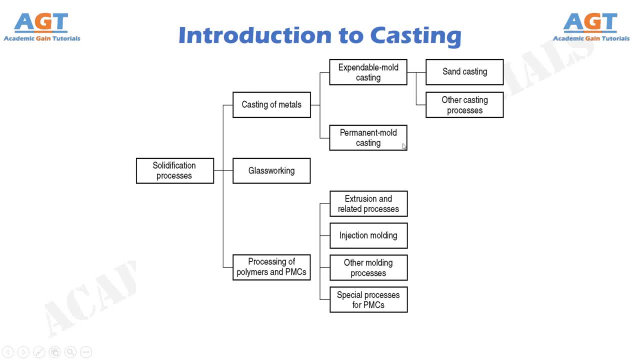 Format is classified as Mustang. type. Brand is classified as The form 세계. In our class we will discuss casting and molding processes. The progressive casting process is classified as expandable mold castings and permanent mold castings. The expandable mold casting processes can be further classified into other casting processes, including the sand casting process. 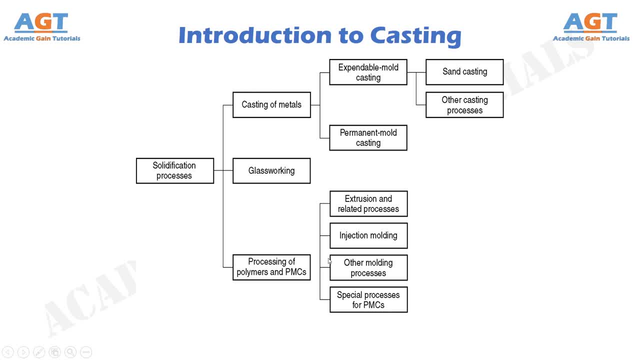 The processing of polymers and PMCs can also be classified into further types, But in our class our topic is to study casting, So we will study everything related to casting processes only. Casting is the process in which mold and metal form and Documenting occurs in different types of casting. 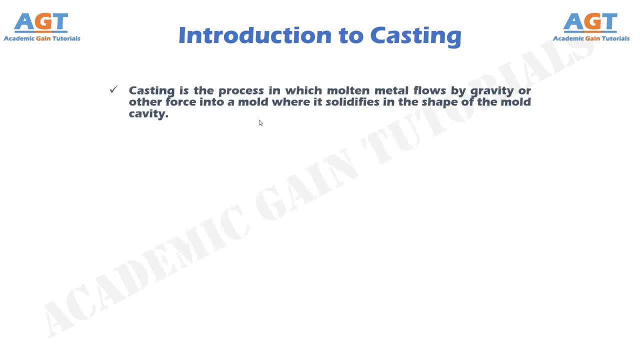 In this classroom we shall consider casting in all cavities, But there is still a certain category based on casting. Metal flows by gravity or other force into a mold where it solidifies in the shape of the mold cavity. The term casting is also applied to the part that is made by this process. 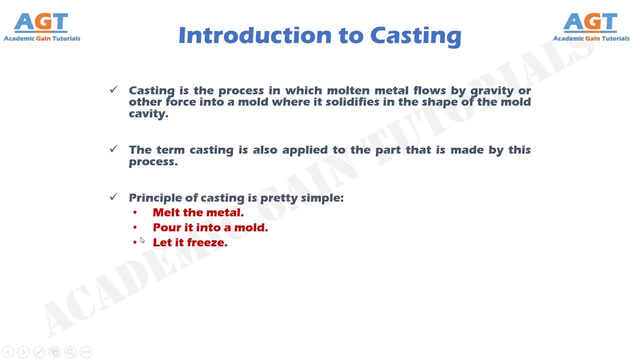 Principle of casting is pretty simple: Melt the metal, Pour it into a mold, Let it freeze. However, to accomplish a successful casting, many variables and factors must be considered. Casting include both the casting of ingots and the casting of shapes.